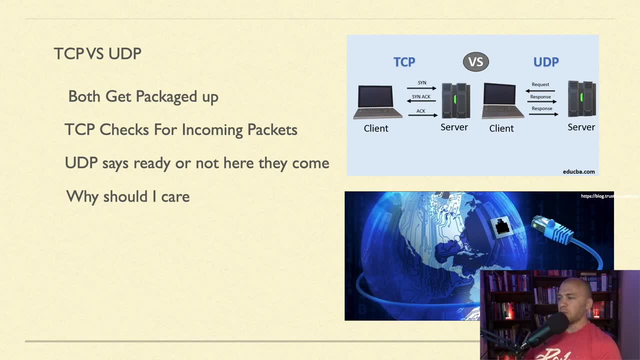 and then the communication will begin to flow between the client and the server. and you're going to see this in the future and you're going to hear it. you're going to have have this question come up: what is tcpip? and so now you know, it's the syn, the syn act. it's the syn, the syn act. 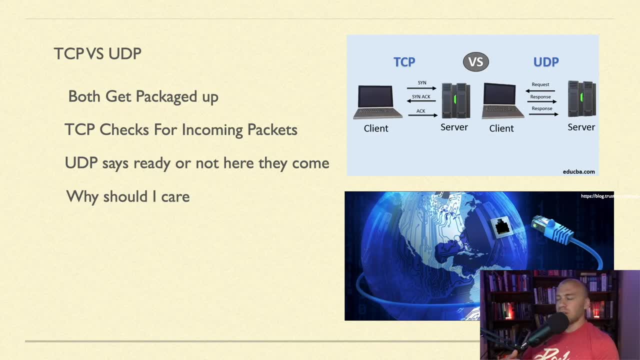 and the act. so it's called the three-way handshake and you will hear this again. so the udp: it just has a request, it sends out the request and it just sends out the response. so what the udp does is it has information it wants to send, it packages it up and it just sends it. some of the packets can: 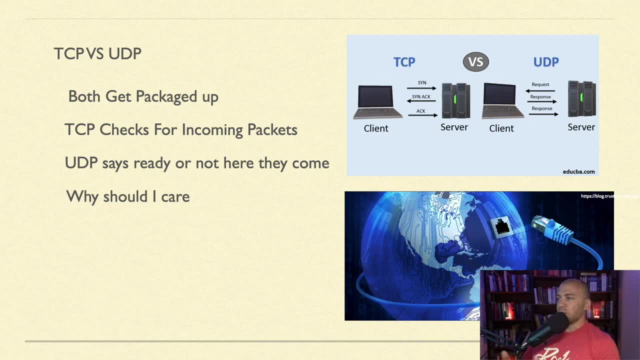 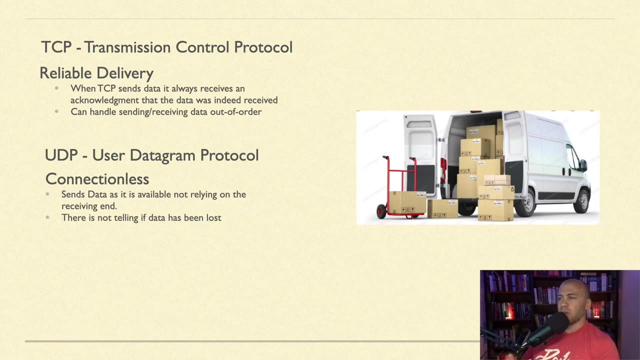 get lost. it doesn't really care what the server or the recipient of the information is has going on, it just sends the information. so you're going to see tcp quite often. the next slide, tcp. we already talked a little bit about the transmission control protocol, what it is, the it's. it's viewed typically as the reliable delivery. 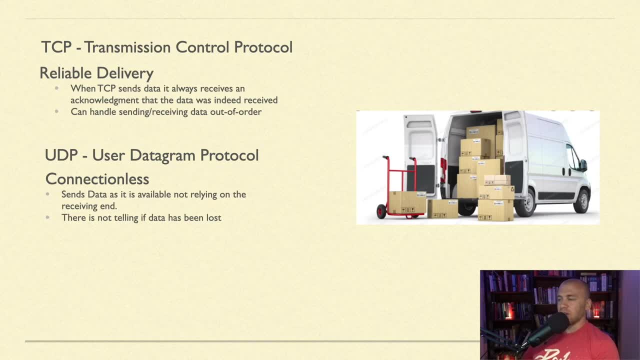 when tcp sends data it always receives the acknowledgement that the data was indeed received. so if some packets get lost, the sender will actually know: okay, some packets was lost. tcp can also handle getting data out of order, and so it can work organize the boxes as they show up. i put the picture in here of a mail truck with the packaged up blocks. 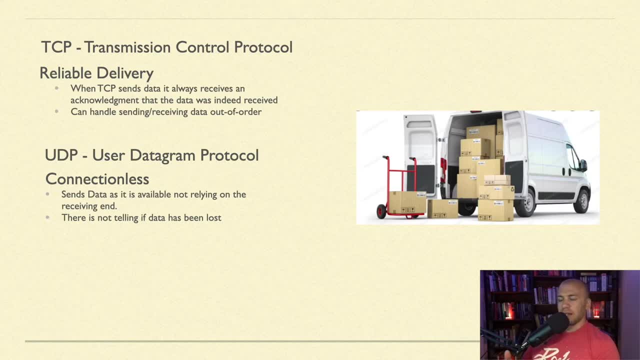 boxes, because this is what it's like when data gets sent. it gets packaged up and then it goes through the network to the recipient, so and then the boxes are unboxed and it can handle getting the boxes out of order. so udp, we talked about this. it's connectionless, it sends data and it. 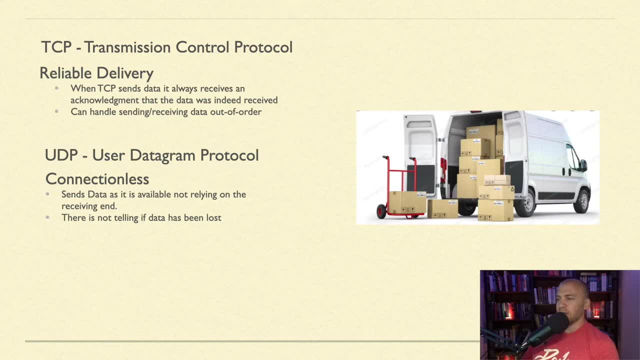 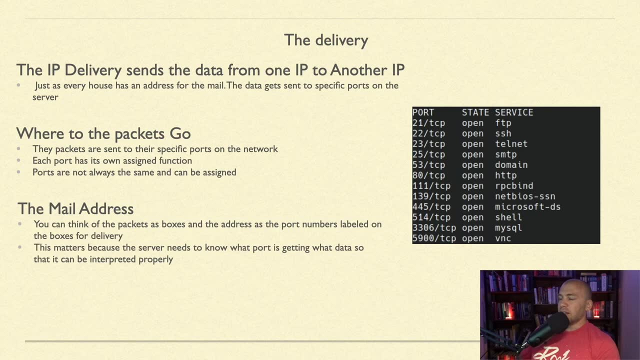 sends it as it's about, as it's available, not relying on the receiving end. it just sends the data. if there's a problem, it just sends the data and then it goes through the network and it just loses data. then it is lost data. the delivery, the ip delivery, sends the data from one ip to 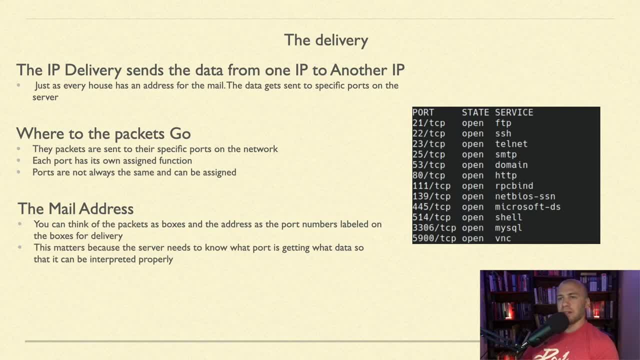 another ip. so, as you think about the common analogy, for this is a house, like you have a house and you have different rooms and you tell one of your children: hey, can you go to this room and get my watch? they have the data, get the watch and then they have the location, which is the room. 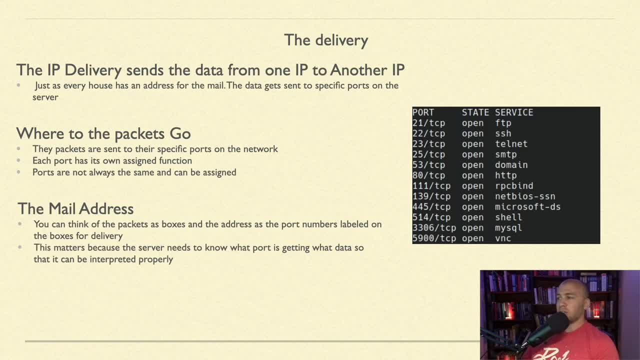 and then they go to the room, they get the watch. so when you think of it like this, you have the data, you have the location, you have the security, you have the information, you have the security, you have the information, you have the security. and so when you think of it in the world of cyber security, you can think of ports. so we 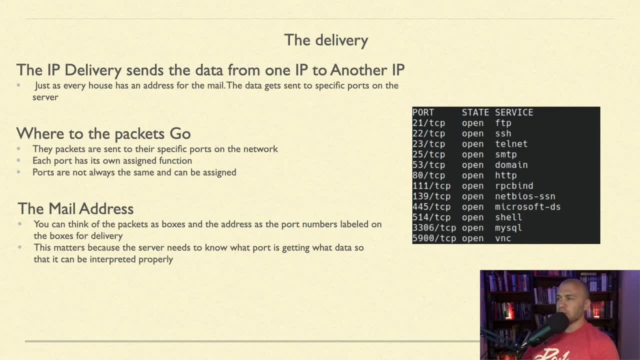 have a image of ports here. the ports are the rooms that are going to be receiving the data. so you tell the. you would tell the server like, hey, i want to connect to ftp and you're going to. it's going to ask you for the data, a login, and then it will go to specifically that port on that server. 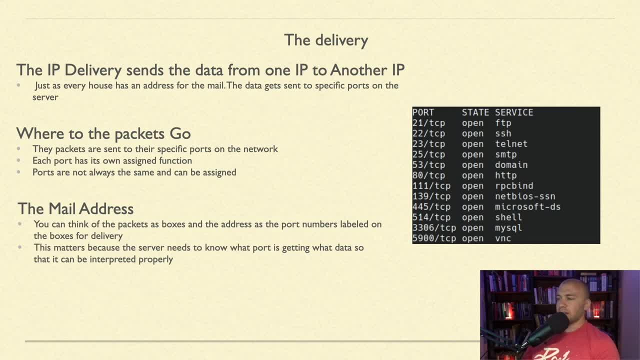 and it will try to communicate. so that's how the delivery system works. so you can see it's a works with the port and so when you, when you want to connect to a port in tcp, it will go out and see if the port is open before it even tries to connect. where to the packets go? that is supposed. 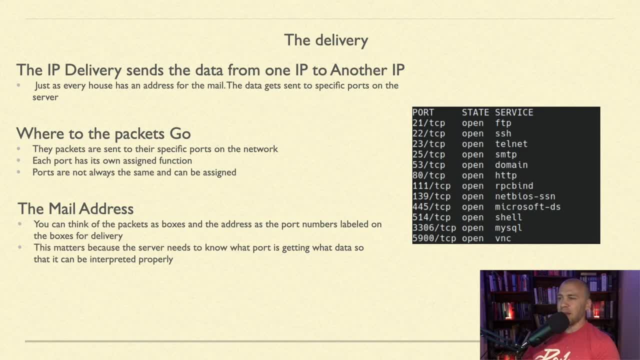 to be? where do the packets go? i have a typo. the packets are sent to their specific ports on the network. each port has its own assigned function. ports are not always the same and can be assigned so each of the ports. you don't want to be trying to send an http request to port 22 because it's. 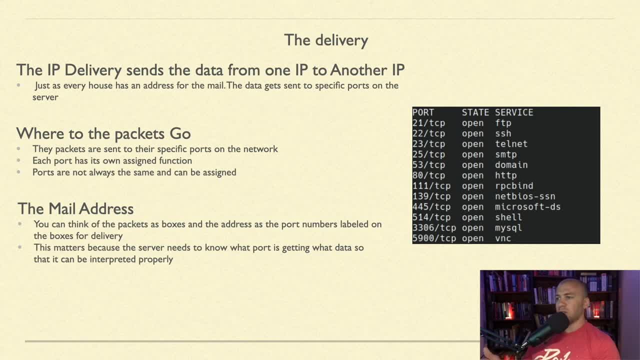 just not going to work. so you actually, when you send out the request, it goes to the specific port, which is running specific programs to interpret the data the way that it is supposed to be sent, and so each port has a specific function. in this scan we have the most common ports that are labeled: 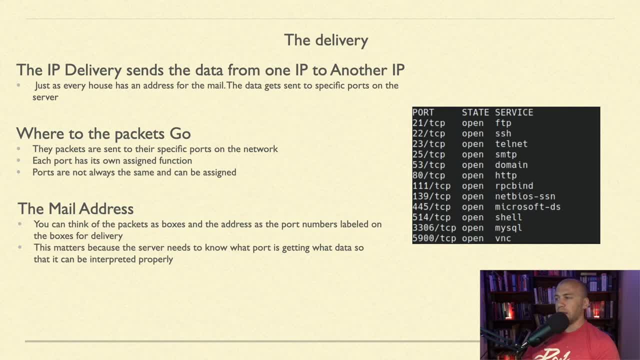 but you can actually assign like http to port 80, you, 81 or 8080 or other ports. you'll see http running on random ports. sometimes when you run an in-map scan you'll also see things like ssh on port 2222, so you can assign ssh to different ports. they. 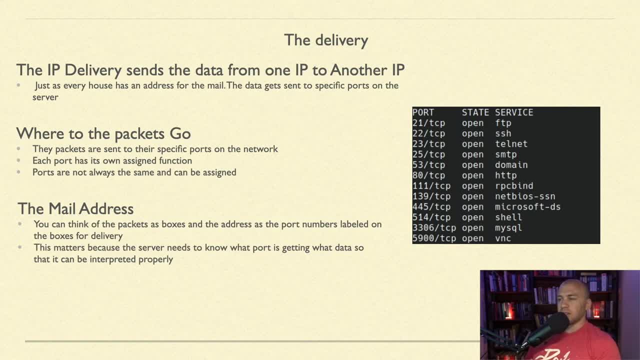 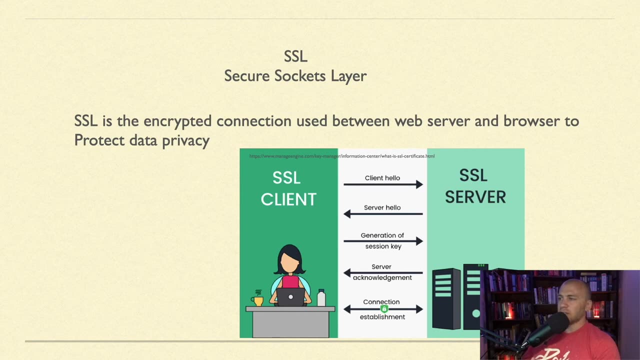 don't always have to be these specific ports and you will see that in the future and so when you. we already talked about the mail address a little bit earlier, so we're going to skip that. the ssl secure sockets layer. ssl is an encrypted connection used between web servers and browsers to protect data privacy. 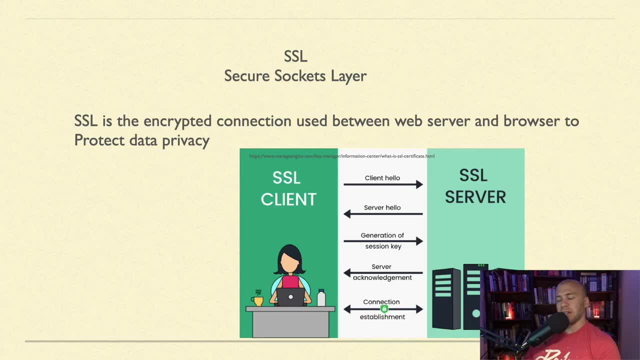 so it tells us exactly how this works. we have this secure socket layer. you're going to see this again. it's going to come up specifically when you encounter a job interview or something of that nature. so this image tells you kind of what happens. the client sends out a request to the server. 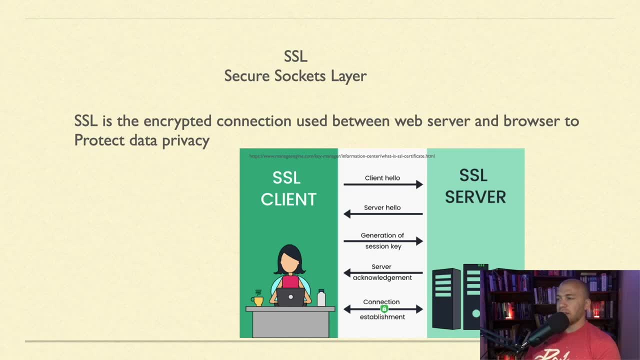 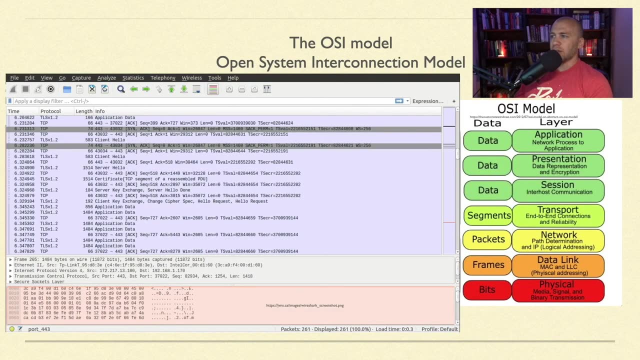 the server acknowledges it and then it sends out a session key and then it encrypts the data as it transfers it back and then stores it. anditos massa- and as you can see, is a dramatic increase in ondata- is the back and forth, the osi model, the open system interconnection model. this is something you 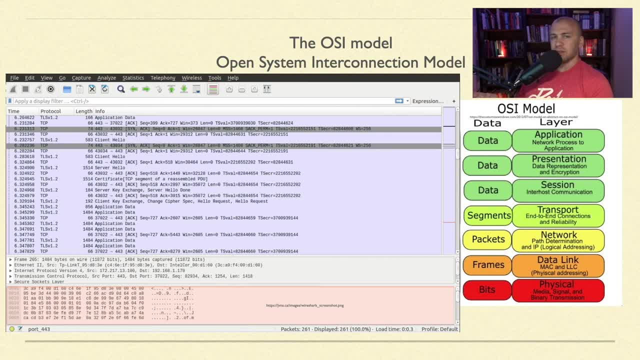 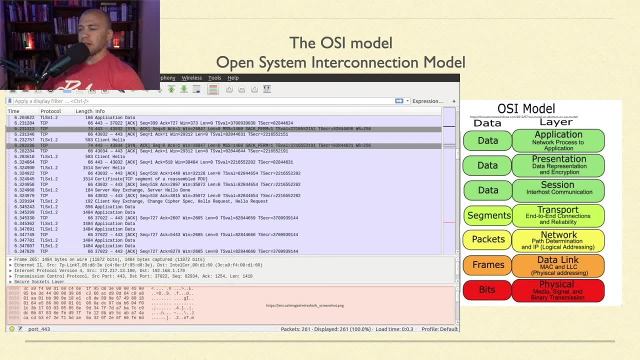 are going to need to know, especially when you're going to be going through a job interview. this is definitely going to come up. this is something you'll need to know in order to communicate with blue teamers or the client you've just done a penetration test for, so you have starting at. 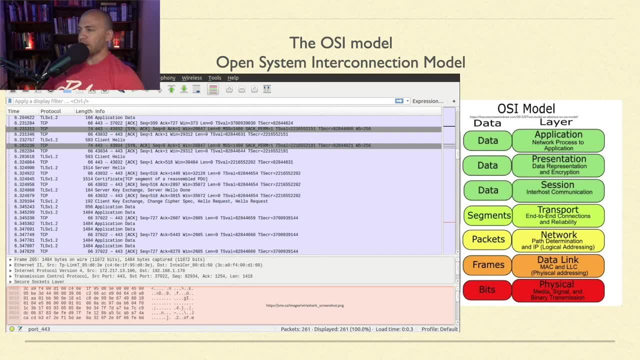 layer one, the physical, and then two and is data, three is network, four is transport, five is session and six is the presentation and seven is the application. so these are the layers and you will need to know these layers. i actually pulled up a wire shark scan here. if you look down where it. 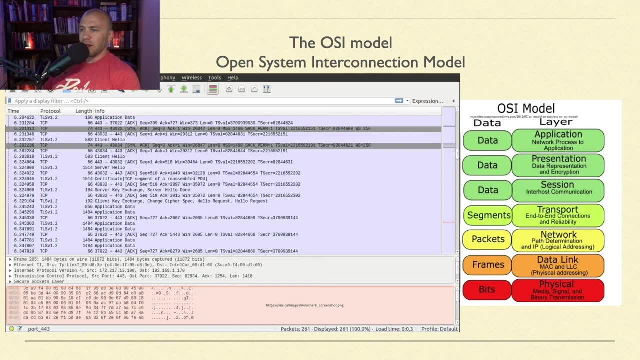 says frame 205, with that little arrow that is going to be your layer one, because it actually tells you what's being sent, and it says here: It's being sent this many bytes- I think it's 1,484 bytes- and it's being sent on a wire. 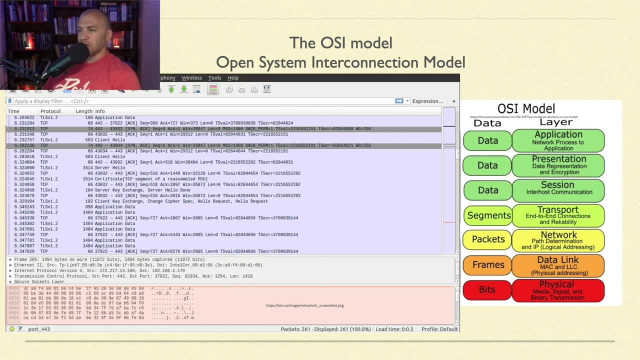 So that is the physical layer on this Wireshark packet, And then the second is the second layer. You can see the MAC addresses there. On the ethernet too, you see both the MAC addresses. So that would be layer two, And then the internet protocol that is being used. 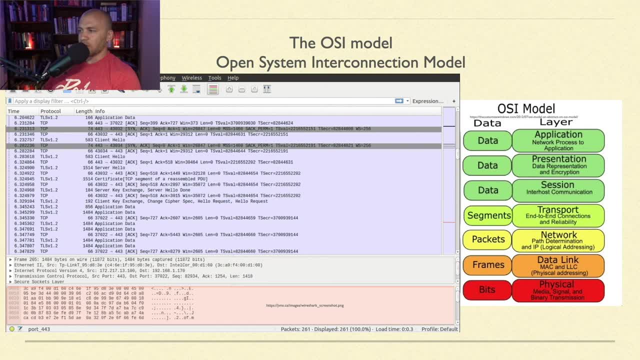 you have the IPs there where the packets are gonna be sent with, And so that's the network layer. And then you have four, which is the transmission control protocol, And you can see the port that is being sent on. And then you have the bottom secure sockets layer. 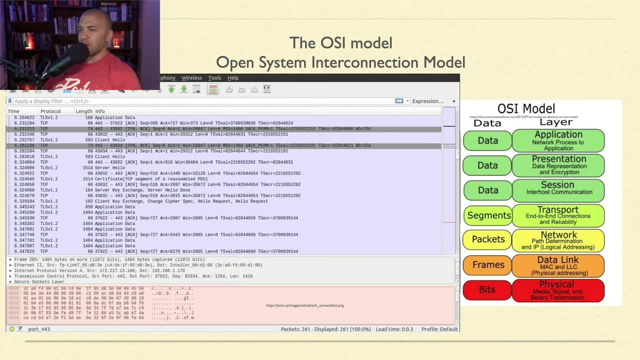 which is gonna be layers five, six and seven, all wrapped up together in that one. So when you look at Wireshark you're gonna be able to see exactly how this works, And so if you find a networking problem, you can say, hey, it's on layer three.